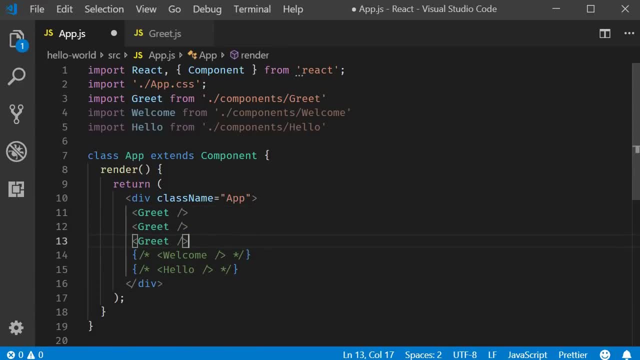 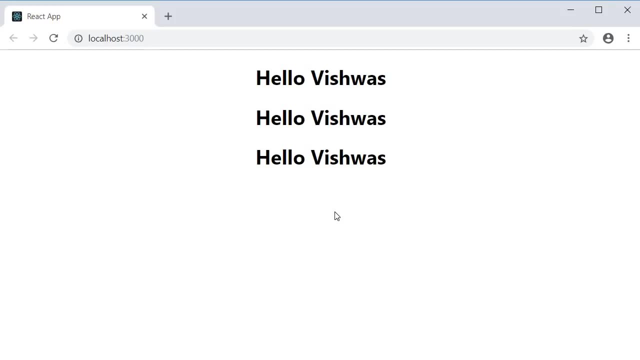 If I duplicate it twice. save the file and take a look at the browser. you can see Hello Vishwas displayed three times. Now this isn't really helpful, is it? What would be great is if we could pass in the name of the person we wanted to greet. 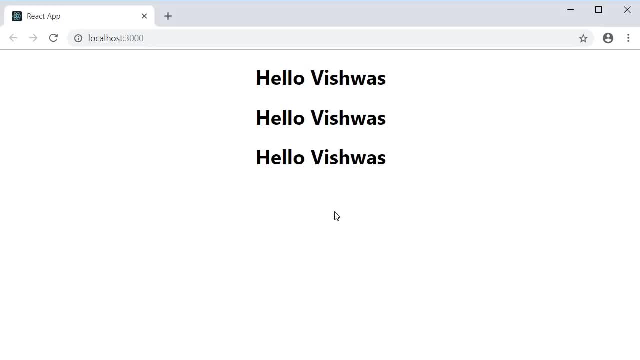 That way, reusing the same component, we could greet three different people instead of greeting Vishwas three times. That is where props comes into picture. Props, short for properties, is the optional input that your component can accept. It also allows the component to be dynamic. 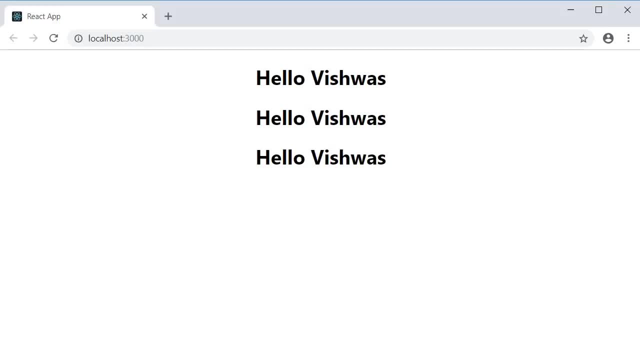 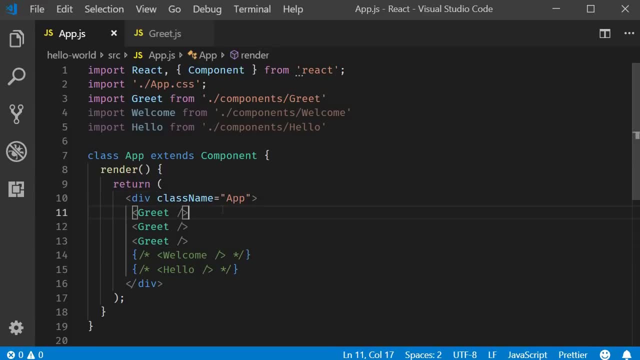 Let's understand how props work in this video. Our intention here is to pass a name from app component to the grid component and render that name in the browser. To specify props for a component, we specify them as attributes. To specify a name property, we simply add the name attribute. 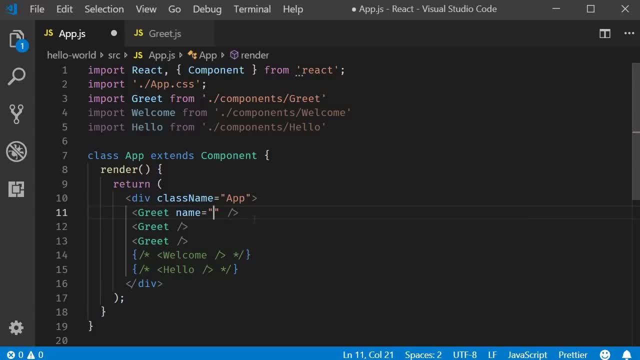 To the attribute we assign the value. Let's go with the name Bruce. Similarly, let's add the attribute on the other two components as well: Name is equal to Clark and name is equal to Diana. Okay, so now we are sending some information or some property to the grid component. 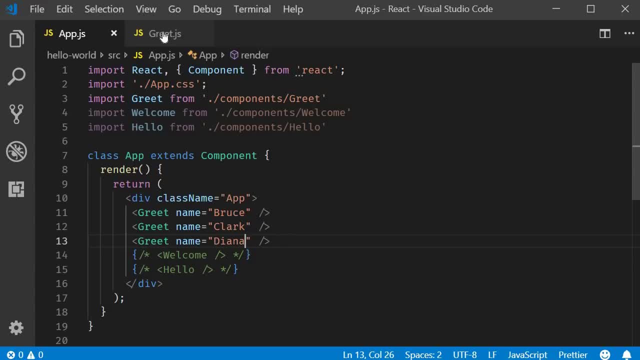 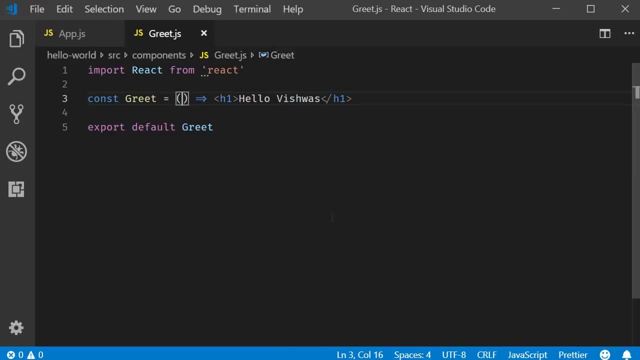 But how do we retrieve these values in the grid component? That is a quick two-step process. The first step: add a parameter to the functional component. You are going to call it props. You can actually name this anything you want to, but the convention is to name it props. 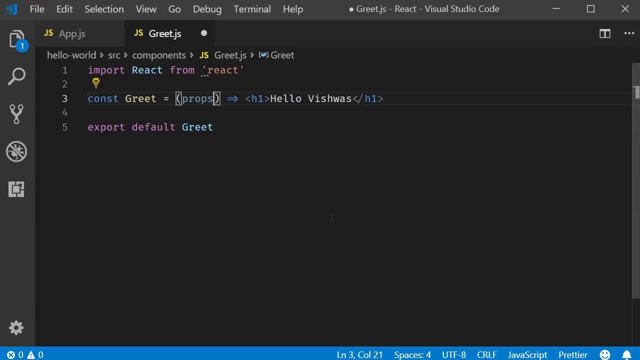 And I highly recommend you don't deviate from this. The second step is to use this parameter in the function body. Now in the function body, let me first log the props parameter in the console. The function body is going to take up more than one line, so we need curly braces and 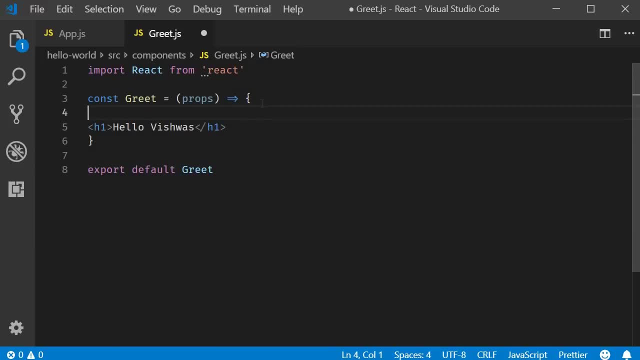 also the return statement, Console dot log props, and then we return the h1 element- Again the necessity of curly braces- and the return keyword is an ES6 attribute. So we are going to use this arrow function concept. If you are struggling to understand, please read up on arrow functions and then continue. 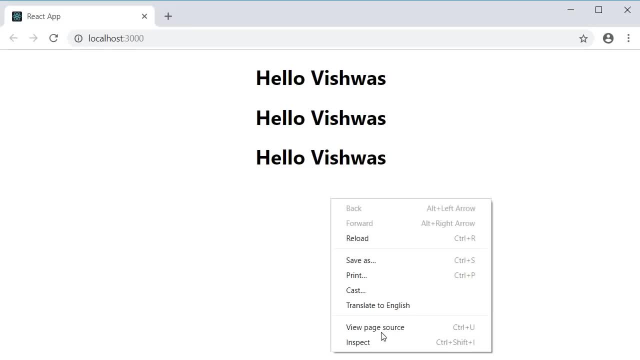 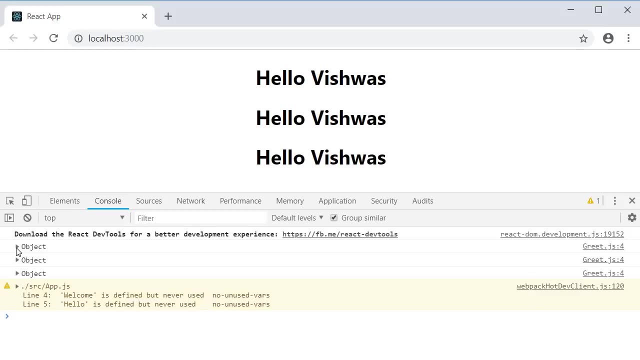 All right. so if you go back to the browser and open DevTools, you can see that there is an object logged in the console. If I expand, you can see that the object has a property called name and a value of Bruce. Similarly, we have Clark and Diana. 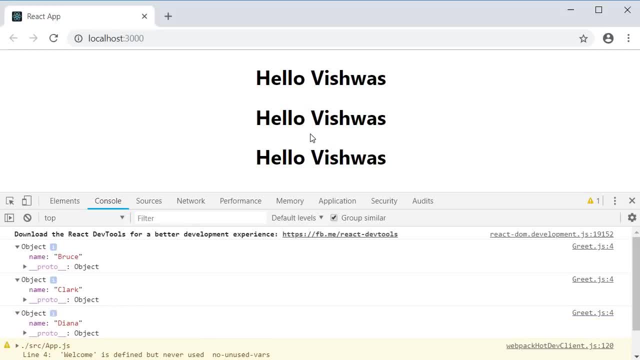 Okay, We have three objects corresponding to the three components. So props is just an object that contains the attributes and their values which have been passed from the parent component. So if you want to display the name that has been passed to the greet component, we need. 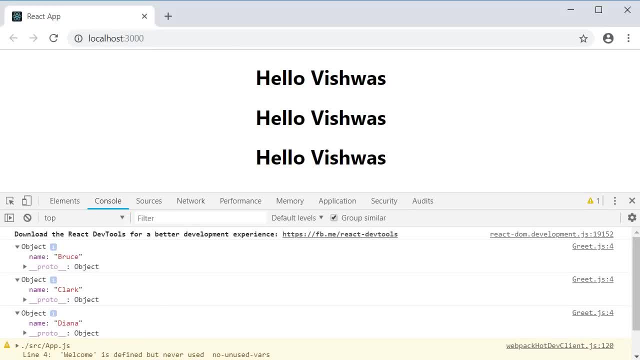 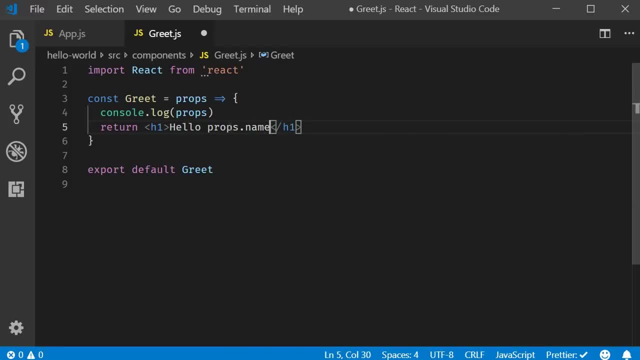 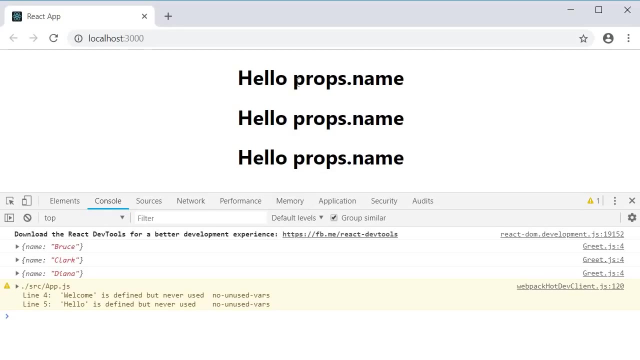 to use props dot name. So back in VS code, instead of Vishwas we need to use props dot name. We save the file and take a look at the browser. The output is not quite what we want it to be and that is because it is being treated. 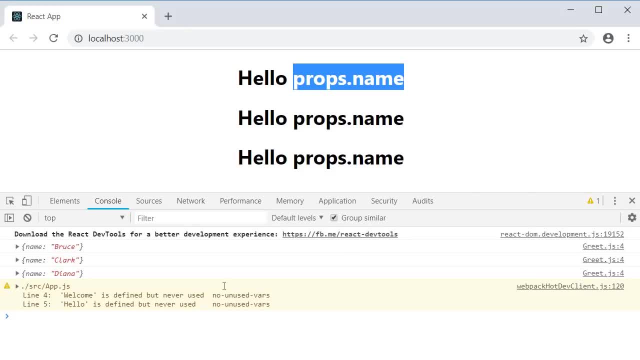 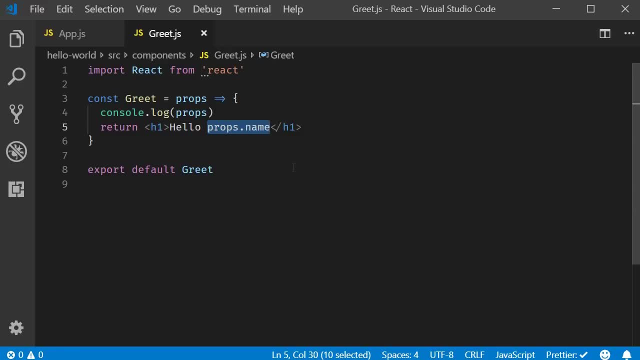 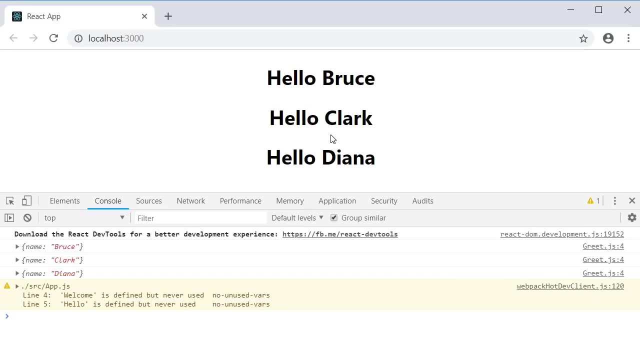 as text. We need to instead ask React to evaluate the JSX expression, and we do that by wrapping the expression with curly braces. The curly braces is a feature of JSX which is really helpful and is used a lot in React applications. If we now take a look at the browser, you should be able to see: hello, Bruce, hello. 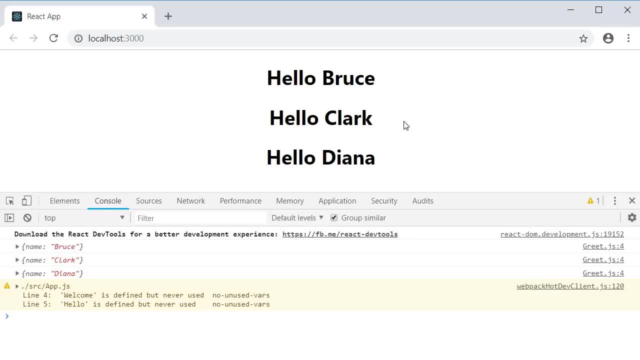 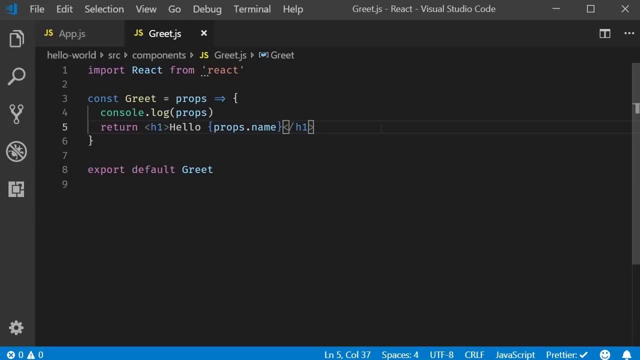 Clark and hello Diana. The reusability of components makes much more sense now that we understand props. Each component can have an HTML template and we can pass in the data we want the component to use. Now let's add another prop to make sure we get a good understanding of how it works. 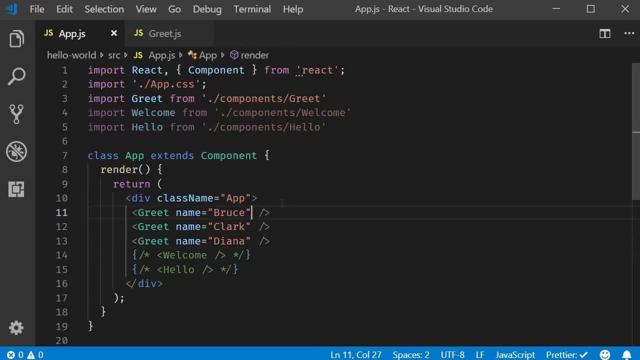 I am going to add a second attribute and I am going to call it heroName. For Bruce, the value is going to be Batman, For Clark it is going to be Superman and for Diana we are going to have Wonder Woman. Now in the greet component, I am going to modify the h1 tag to hello props dot name. 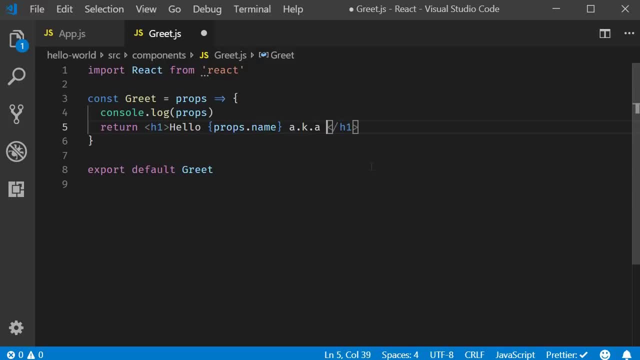 aka also known as within curly braces, props dot heroName. Now I am going to add a second attribute. I am going to call this heroName For Bruce this value is going to be Batman. For Clark, this value is going to be Superman. 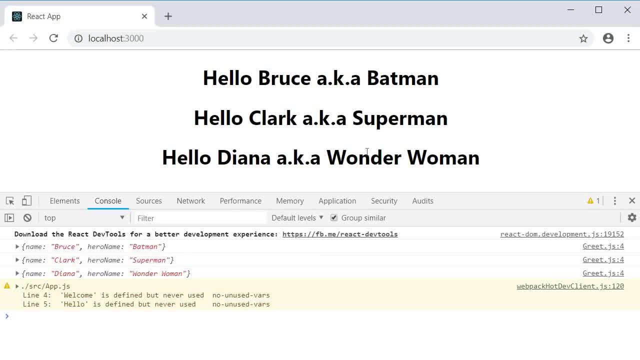 Now, if we take a look at the browser, you can see that the output is what we expect it to be. Sometimes it is also possible that you might not have an idea as to what content is being passed in, but we want the component to render that unknown content. 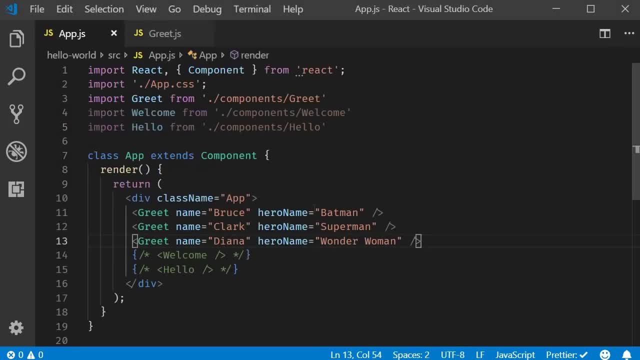 We can do that by specifying the content between the opening and closing tag of the component and retrieving it using the reserved children property in the props object. Let's understand better with an example On the first grid component, instead of the self-closing tag I will split it into opening. 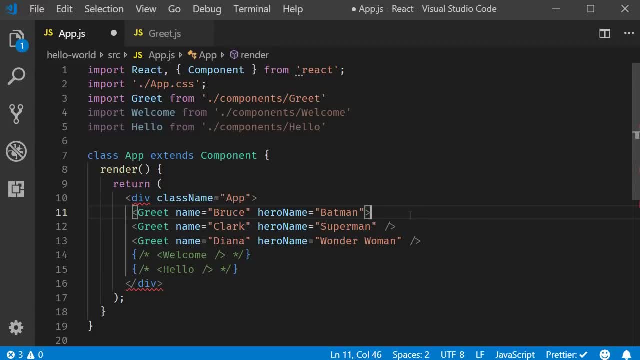 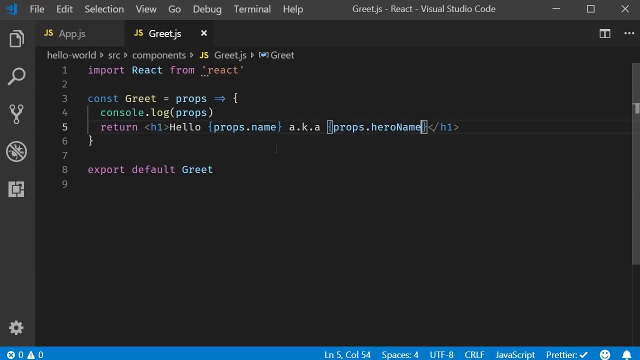 and closing tags. In between the tags I will specify a simple paragraph tag. This is children- prop. Now in the grid component we can render that paragraph using propschildren. So first I am going to be adding parentheses, as I will be splitting the JSX into multiple. 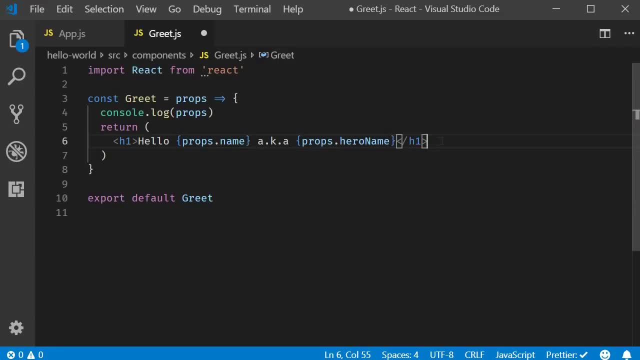 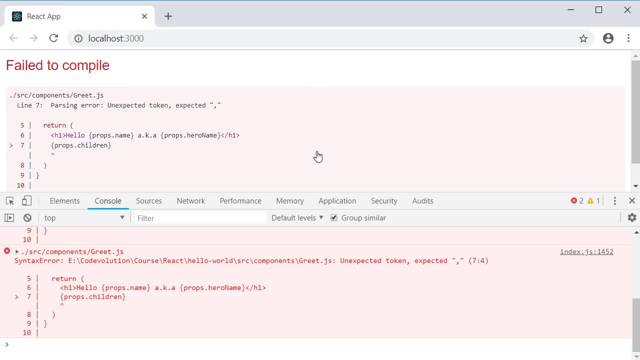 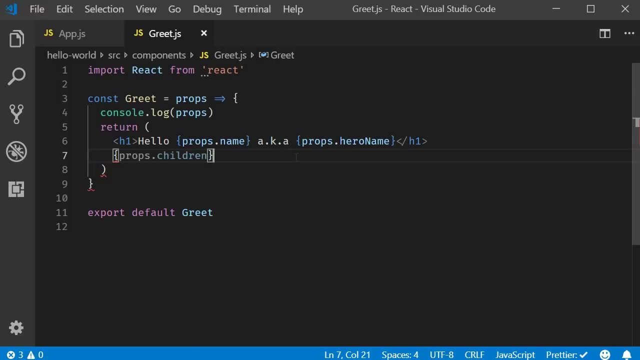 lines. The first line is the h1 tag and then, within curly braces, I will add propschildren. If I save the file and take a look at the browser, You can see that we have an error. This is because the JSX we have should contain only one wrapper element. 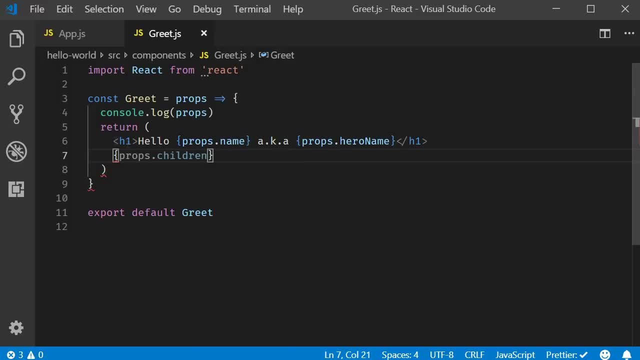 So, back in VS Code, we are going to wrap both these elements within a div tag. So this is a limitation we currently have. We can return only one HTML element, So we have to enclose all our content in one div wrapper tag. 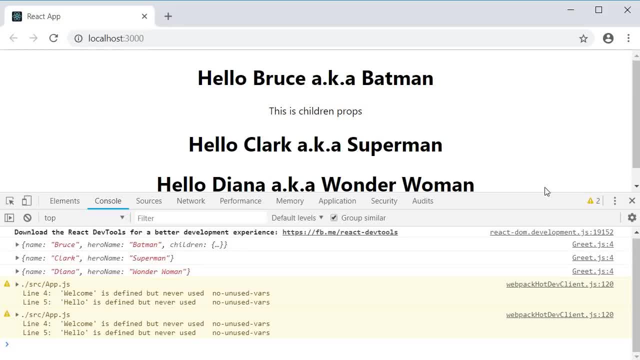 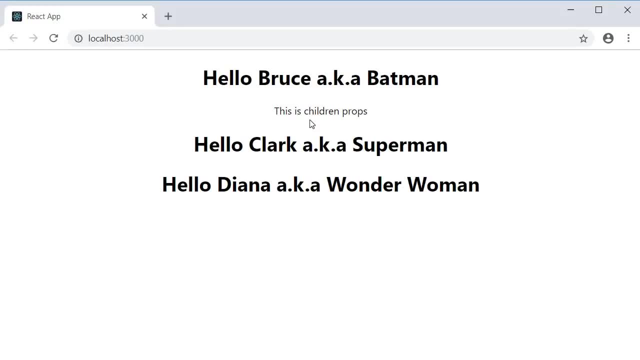 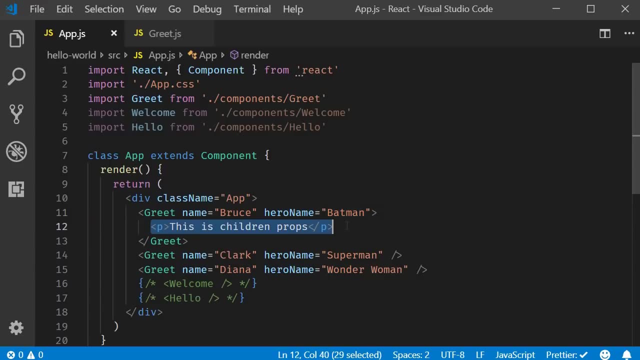 If we now save the file and take a look at the browser, You can see that only for Batman we have the additional content being rendered. This paragraph corresponds to the inner HTML of the grid component- This right here. So if I were to add a button tag to the second grid component? 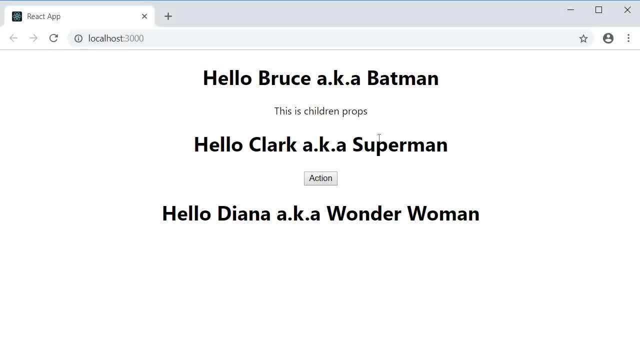 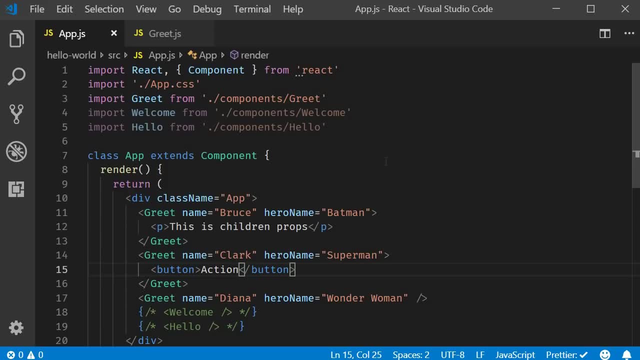 I can add a button tag to the third grid component And take a look at the browser. The button should be rendered for Superman. So for the properties you know for sure are going to be passed. you can pass them as attributes If you have no clue what is going to be passed as props or if you have to pass in dynamic. 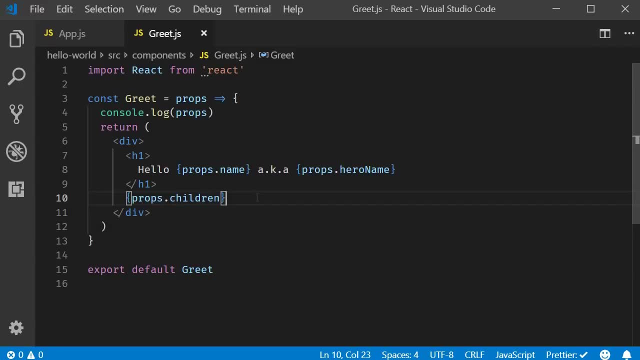 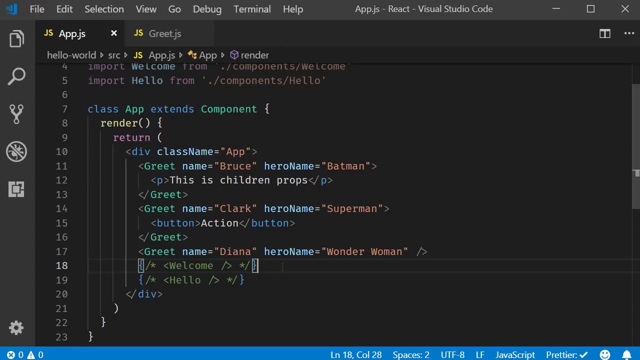 HTML content. You can use propschildren. If at all something is specified, it is rendered in the browser, And if nothing is passed, propschildren simply renders nothing. Next, let's see how to make use of props with a class component. Now, irrespective of the component type, the properties are mentioned as attributes during. 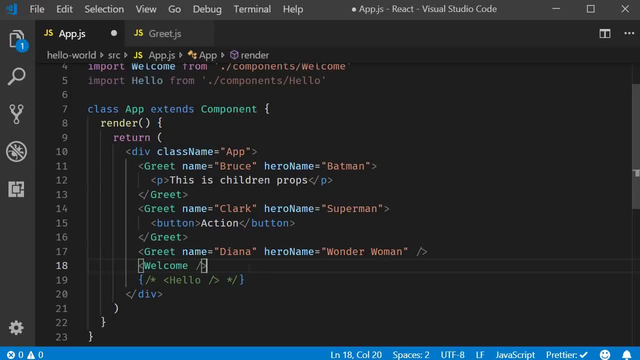 the component invocation. So we have our welcome component, Which is a class component, And I am going to duplicate it twice. Next, I am going to add the exact same attributes On the first welcome component: name: Bruce and hero name: Batman. Similarly, Clark and Diana. 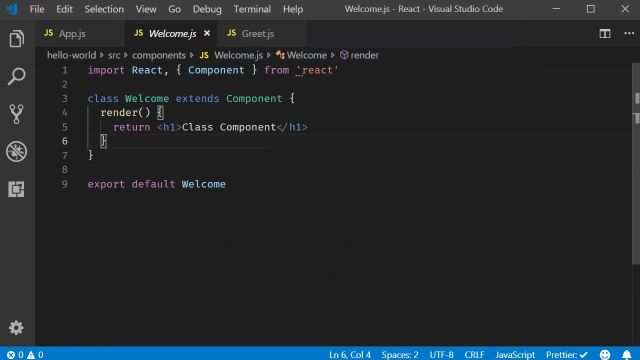 Now in the welcome component, let's use these values. Unlike the functional component, where we specify the props parameter in a class component, the properties are available Through thisprops, which is reserved in class components. So in the HTML we can have welcome thispropsname, also known as thispropsheroName. 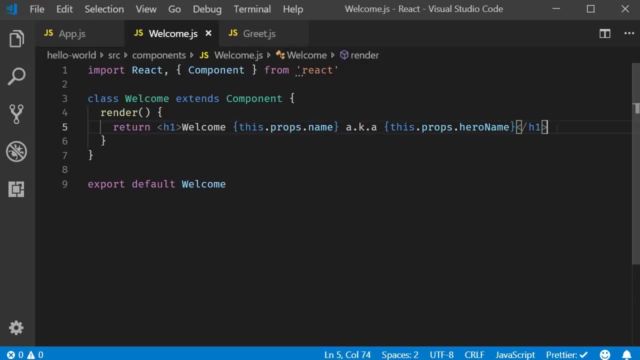 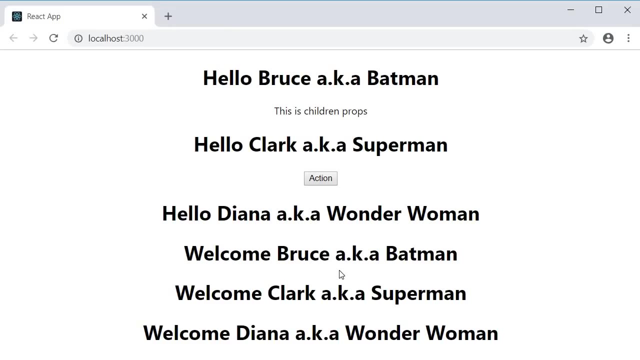 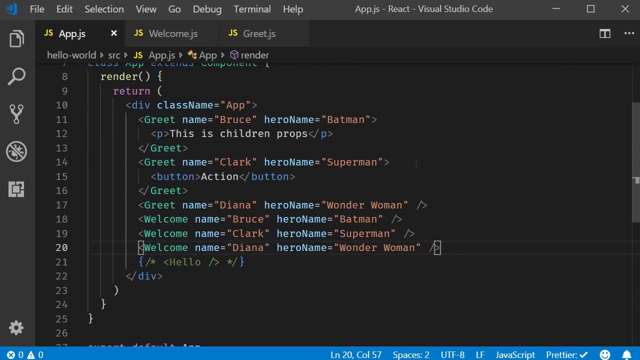 Basically, You are accessing the props with this keyword. If you save the files and take a look at the browser now, You should see the expected output. Welcome Bruce, Clark and Diana. So that is pretty much the basic idea behind props. When specifying the component, you can include additional attributes.